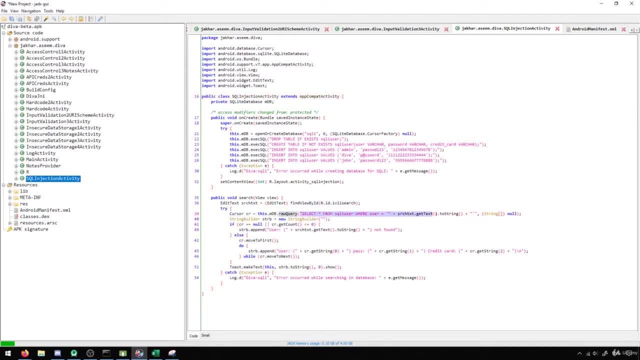 here it's doing a raw query against the database And this is the query that's actually happening And you can actually see that when it encounters an exception it's going to actually show the exception in the error log. So this means that if we go into our log cat, which I've got open here, 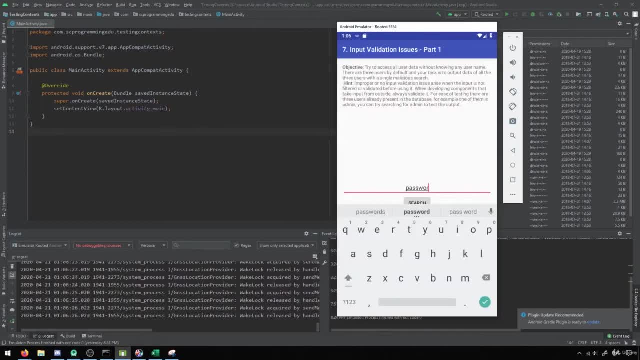 in Android Studio when I input in something invalid. so, for instance, a very good example of this would be like a single quote. a single quote is a piece of SQL syntax. if it's interpreted like code, it should cause an error. You'll see when I search this. we've got this error here that says: 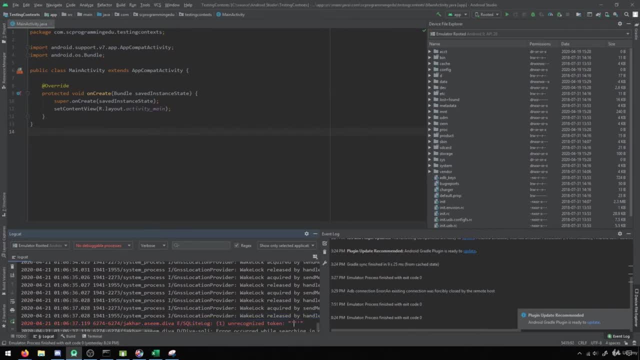 unrecognized token. This tells us that we're interpreting that token as code rather than interpreting it as an input. So this means immediately to me that this is vulnerable to SQL injection. So let's take a look at how we can craft SQL injection with this. we have access to the 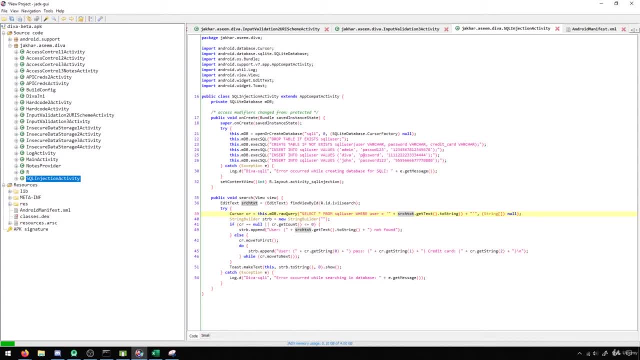 query here And again, this isn't an uncommon thing. if we can decompile the code, we can gain access to the queries And, as you can see, our input is going in right here. So it comes in right in the middle here, right in between two single quotes. What that tells me is that, if I can end, 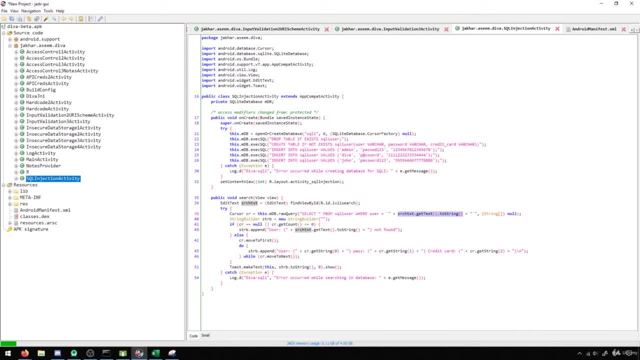 the single quote and then input something that's always true and then maybe put a comment at the end that will allow me to execute where user equals blank, or say one equals one, which is always true, which will return to me the whole database back. So let's take a look at exactly. 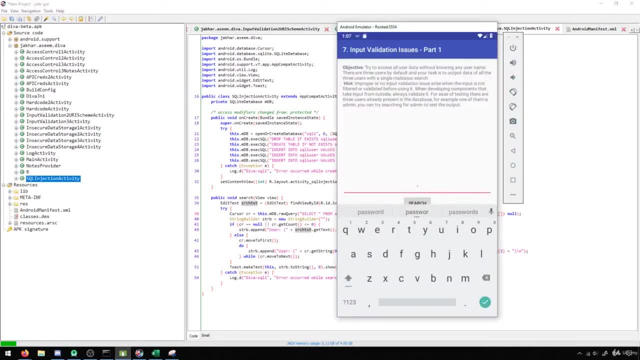 what that looks like. If I put the closing quote here, this will close the users input And then we'll say: or we could say, or one equals one, And then we could put a comment, So those two dashes at the end as a comment, or one equals one is something. 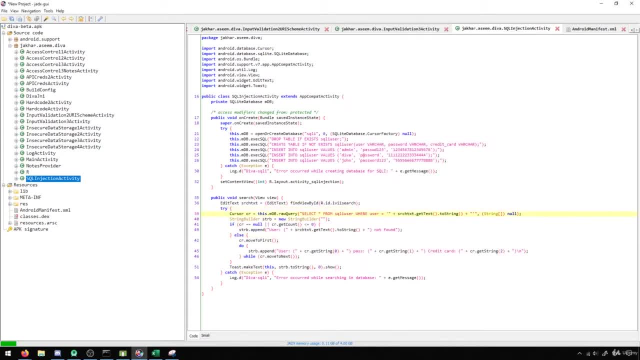 that's always true, And the closing single quote would close off this starting quote here, So it'd be user equals blank or one equals one, And then we comments that this end brace here or this end single quote here is an interpreted as code, And in doing this it will give us a valid query. 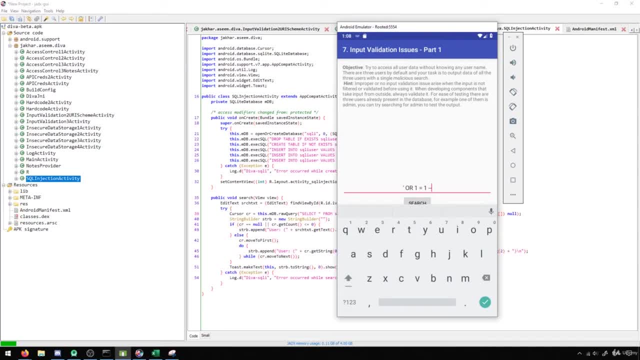 And that valid query is going to return to us all of the contents inside of the database. So you see, when I click Search here, it exposes the whole database credentials, right. So you can see that this is an example of being able to leak information from a database using an invalidated 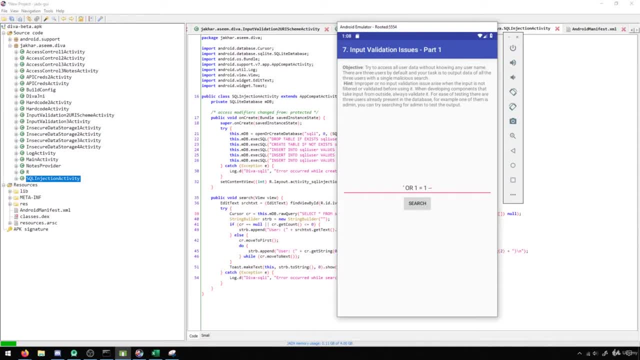 input. So SQL injections are a very common type of input validation error that happens in a lot of different instances. So this would be one example, And this is one thing that you're always able to sort of test. The error is actually printing into the log. it's actually quite rare that someone would give you. 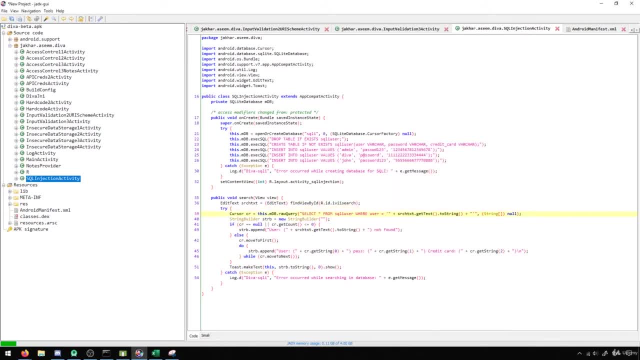 that. However, again, if you just sort of like search for raw query or query in general, you should be able to find instances where this sort of thing happens. So this is one type of input validation that's relatively common. I'm going to show you another type of input validation that is rather 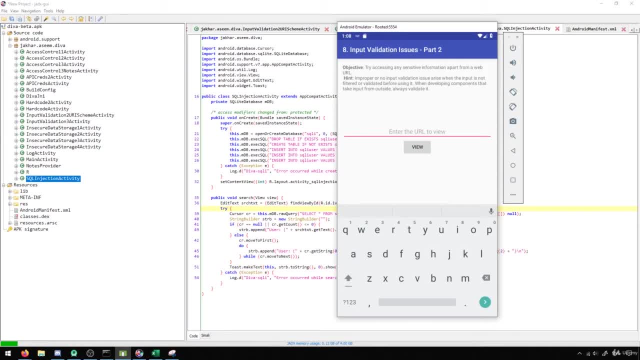 interesting and a little bit different. So with this one here, you see that we can type in a URL to view. So if I put in like Google dot ca, for instance, I press View, you see, it brings up the web page for Google. So this is just like a simple. 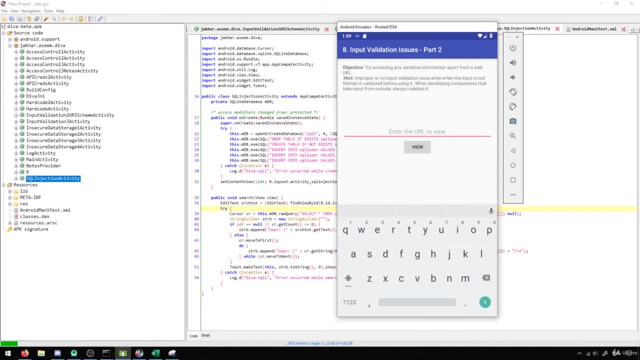 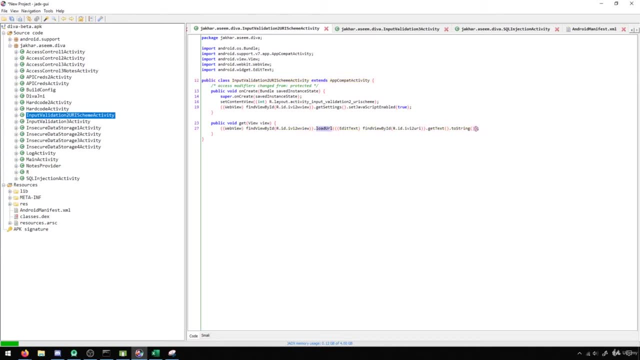 web browser And if we go into the code of it we can get a bit of a better idea of what's actually happening. So you see, here we have the input validation scheme. you see that it just does a load URL. Now, on the surface this probably looks quite innocent, because load URL would imply to us that 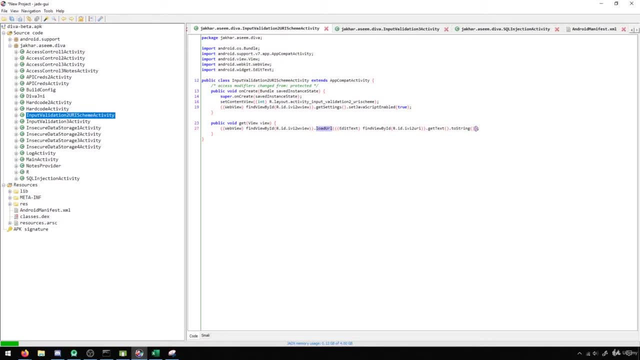 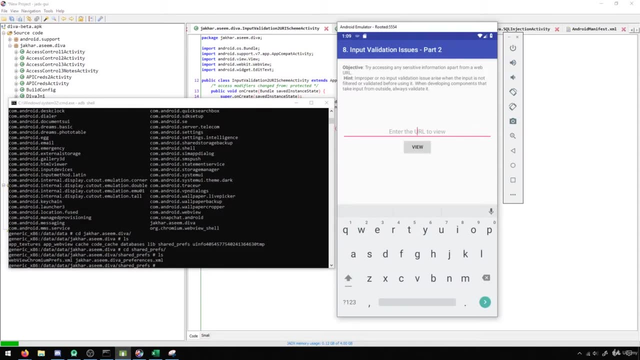 we're just loading any sort of- you know- web page URL. However, the interesting point here is that in Android, we actually treat files as URLs as well, So we can actually access files on the system using the URL path of them. So, for instance, you: 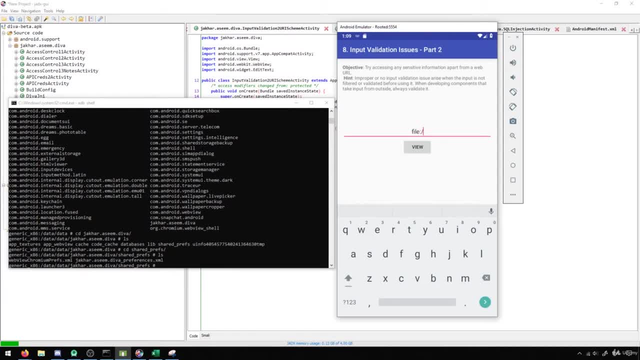 could do something like this: you could say file, you go colon and then you put three backslashes And then you put in the path to the file. So we'll say data, data, for instance. I'm just going to pick a file that I know exists. So 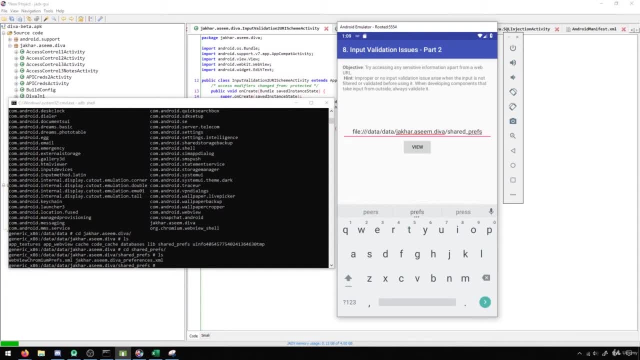 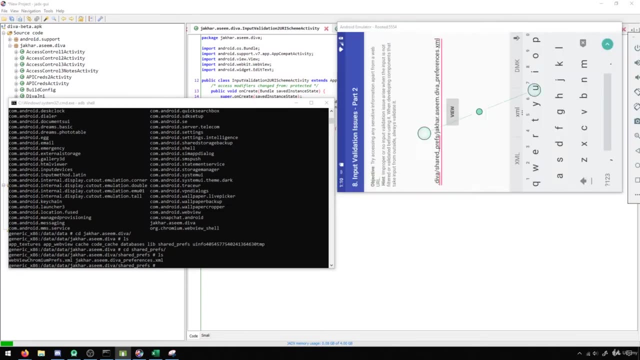 this is inside of the data files that we're looking at. we were taking a look at insecure storage And we know that there's one here called Jakarta seam dot diva underscore preferences dot XML. So you can see- I've just put in the whole path of the of the file. 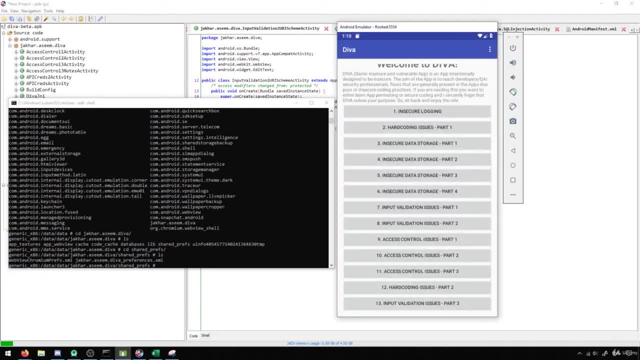 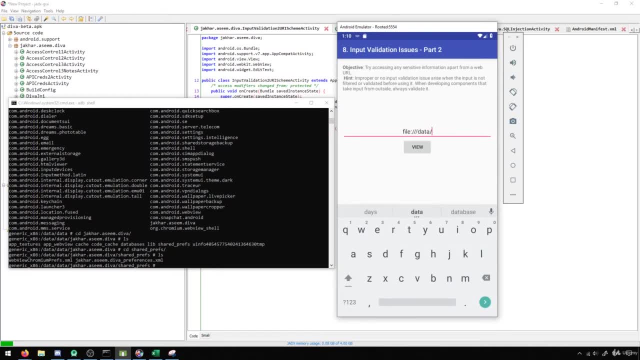 itself And it just crashed there. So let's try that one more time. Not sure why it crashed there. We'll give this another try. Yeah, there are some instances where this app may crash on you. Yeah, it's not overly common, But it could be from some other testing that I was doing related to this app for input validation. But 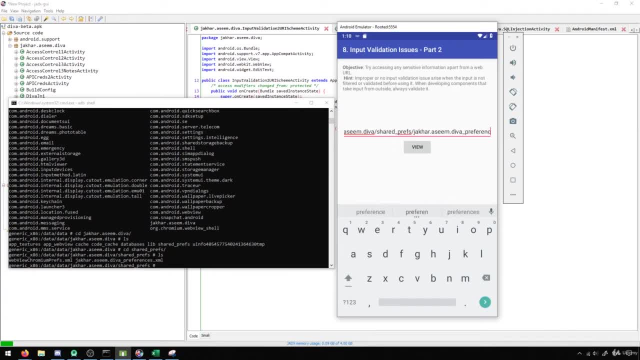 let's go ahead and try this diva preferences dot XML. You'll see, when I click on view here, it actually displays the file below here. So, if you remember, this is the file that we created in the in the improper storage. So this shows us how we can actually access that. 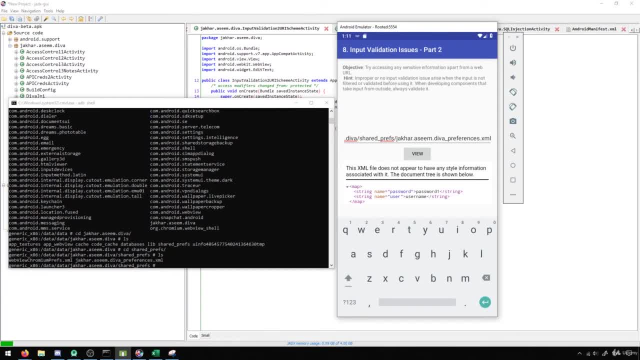 storage, without necessarily even having root permissions. If we happen to know this path, which it wouldn't be unreasonable for us to know it if we have a rooted device, we can find it very easily, or we can find it through the code we can actually access it, if there's ever like a browser that happens to take in these file paths for. 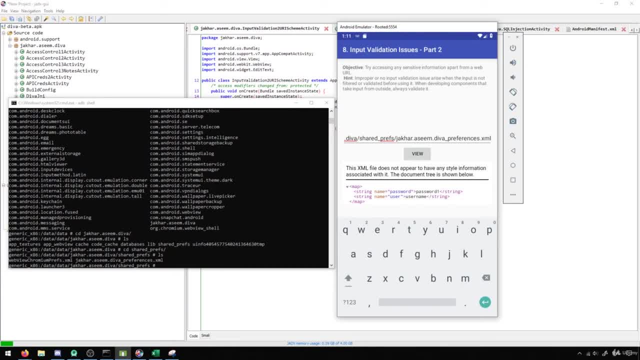 instance. So this is a very critical vulnerability because it allows for information leaks And we can get to really any sort of file on the system utilizing this, And we might even be able to access this from other applications if it has like a provider that allows us to launch this. 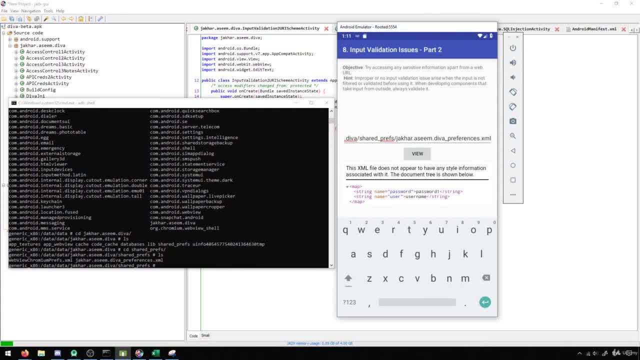 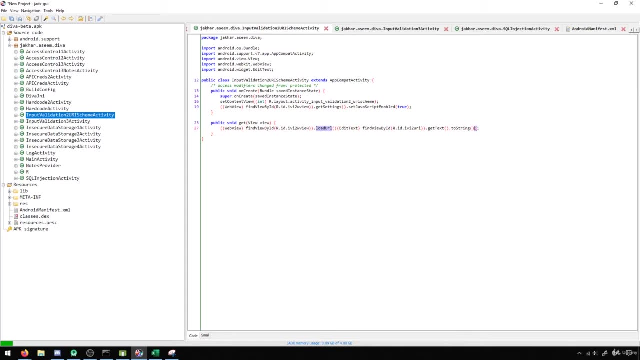 activity maybe right. So This is a very common and critical vulnerability. So this is another type of input validation that you can look out for. So I think it's parsed like a web page. utilizing this load URL, It's very possible that we'll be able to load internal URLs which are actually passed to files. 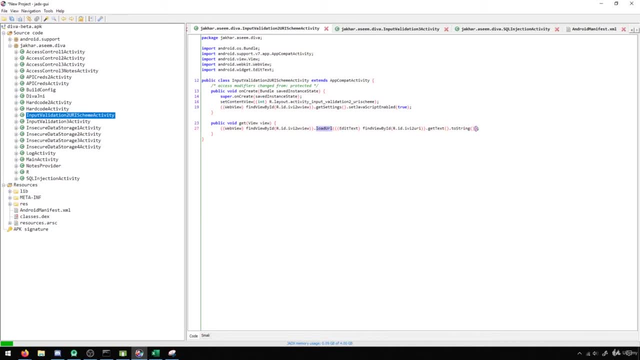 So this is another type of common input validation Again. so we have databases and we have URL loading. The third type of input validation is a little bit different And the way that it essentially works is by calling external libraries. So what you'll see here is this: uses the DJNI, not function but class, rather. 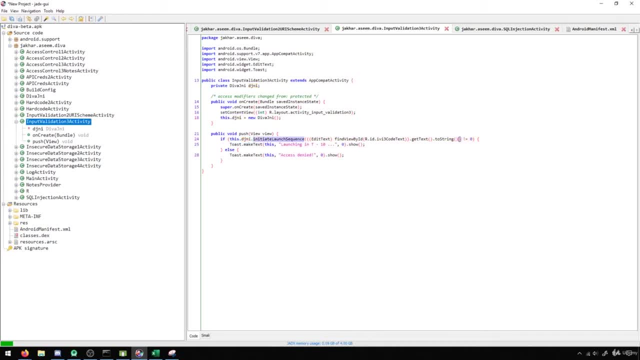 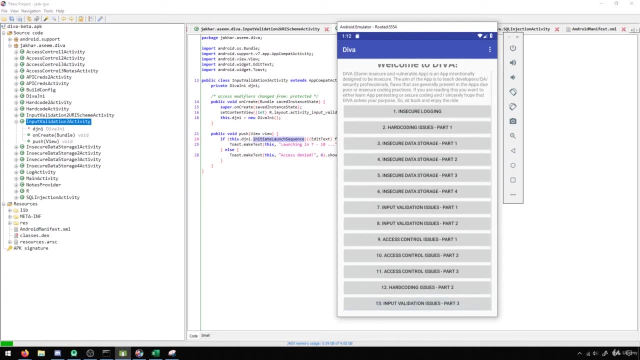 And you see that it uses a very specific piece: initiate launch sequence. So what's interesting about this is that if we go to this input validation three, what we're able to do is we're able to put in some inputs and attempt to get it to launch. 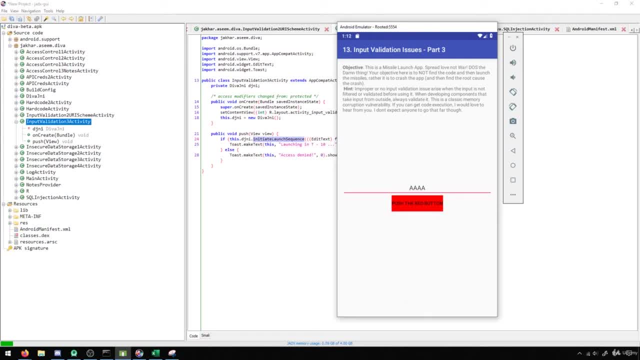 And you'll see, it gets this access denied In these cases. what we're actually able to do with this is, since it's loading a shared object library, it means that it's probably written in C or C++. C and C++ are relatively infamous for buffer overflows. 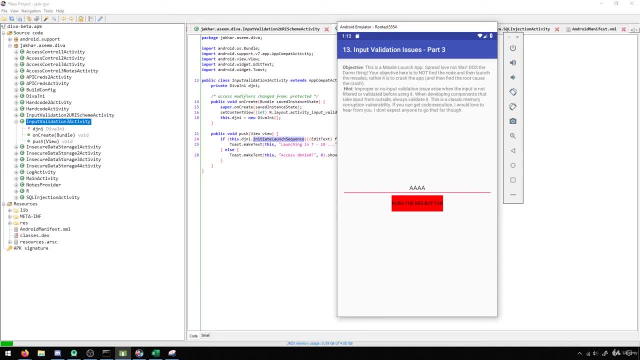 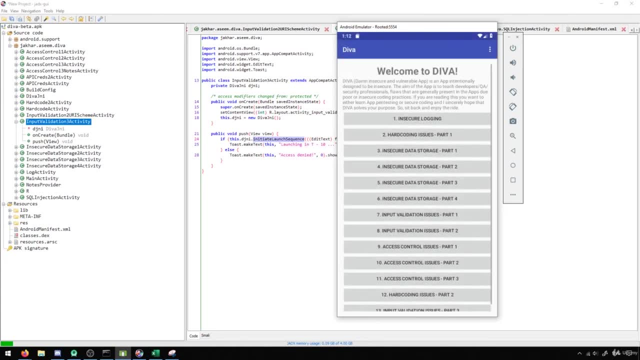 If you can input something way too big into this input, we may be able to get it to overflow. So, for instance, if I just type in like a whole bunch of A's and I push the red button, you'll see the application crashes. 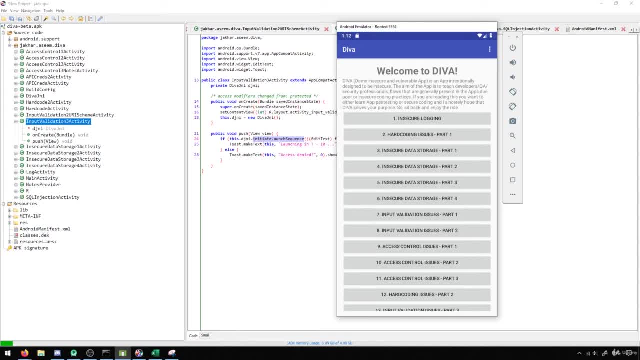 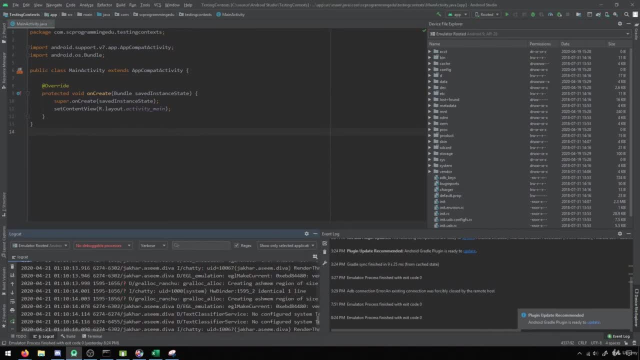 When an application crashes like that, it tells us that there could potentially be a problem And it might be related to a buffer overflow. If we want to get a bit more detail, we can actually go back into the logcat logs And I'm assuming it's probably going to give us some information inside of here when we try to crash this. 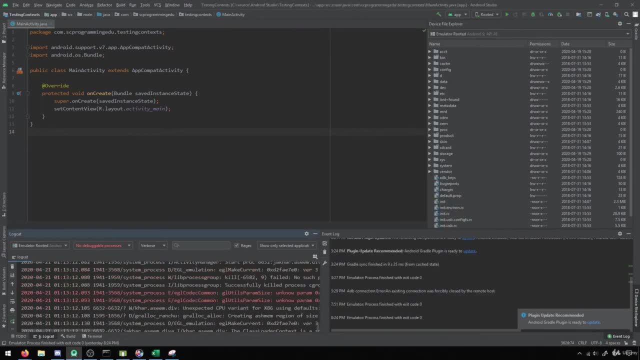 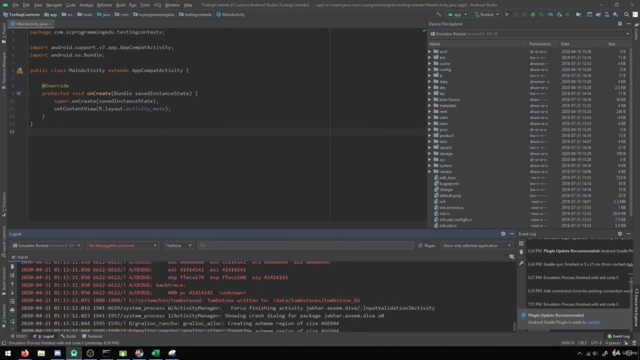 So let's try this again. Yeah, you'll see there we got the whole like sort of dump. So this right here is what we would call a stack trace, essentially So you can see it gives us a lot of information here. The main things that you want to get here is that you see the parts of the stack. 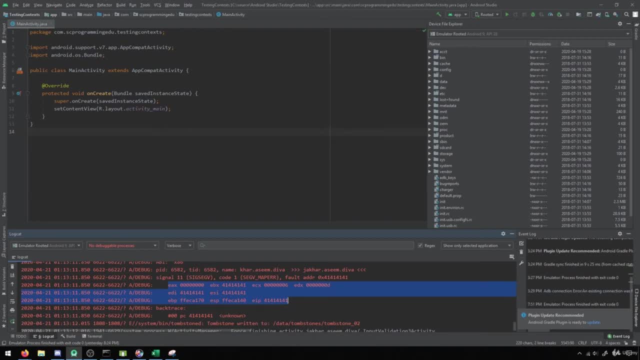 So we can see that we're actually overflowing the stack here, And you can see that it's giving us some errors related to that. Now, what happens here is, if we can actually specially craft our input, we may be able to get the device to execute code. 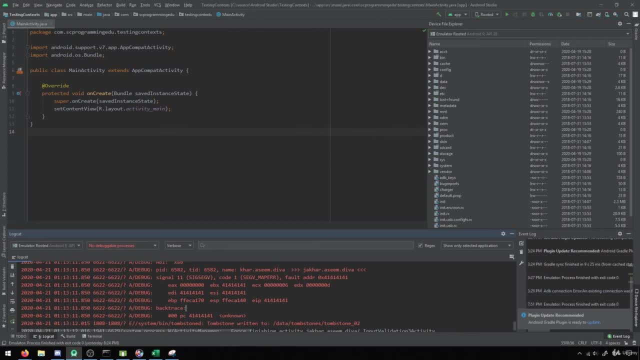 which may be able to get us access to execute code under the permissions of the application itself, And this would be an extremely critical vulnerability. This is like a CVS 10.0.. But even just getting the stack overflowed It's not very useful to happen- creates a very critical vulnerability as well. 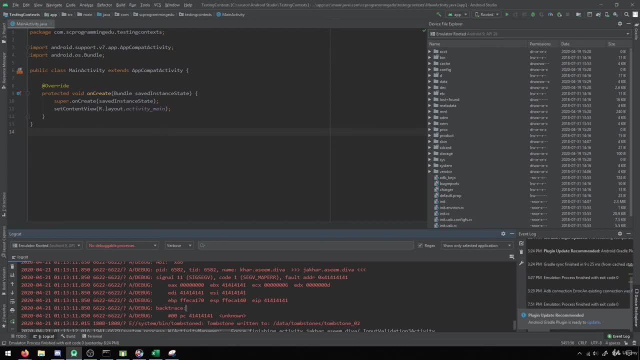 So in oftentimes, like with Java, it's not very common to see a stack overflow, But if you're using C, C++ libraries or languages similar to that, where you have to do memory management, this is definitely something that's in the possibility. 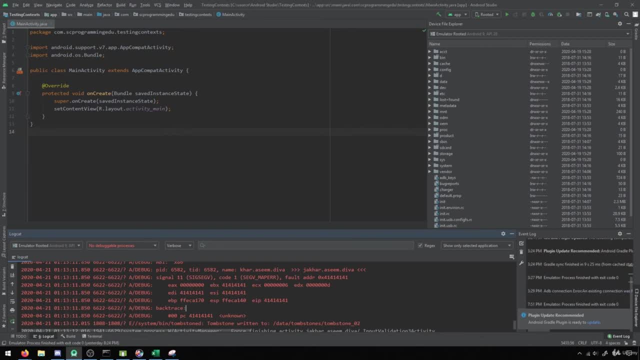 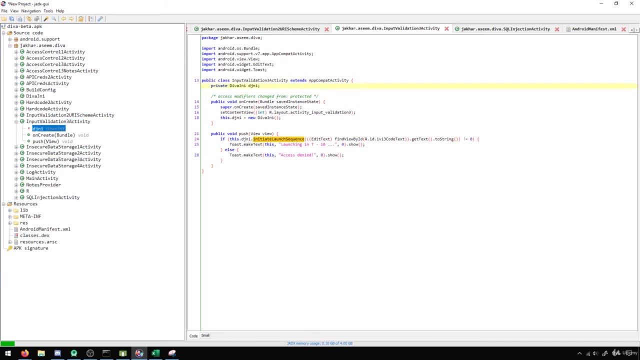 So, if you're able to find something like this, it's an extremely critical vulnerability And, again, the things that you want to look out for for this is any sort of class that is loading a shared object. So this DJNI class- We talked about this earlier.